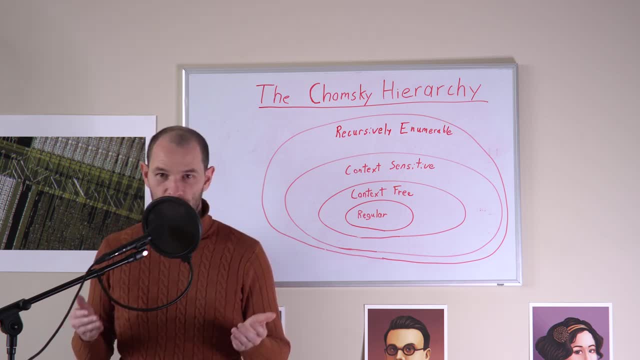 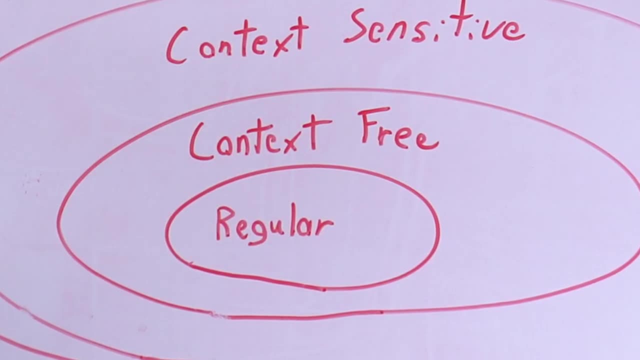 is that it doesn't go far enough. I think that it was an interesting and new perspective back in 1956, but it's really overdue to be replaced by a much stronger and much more useful model. I do think that the distinction that's made between regular languages and 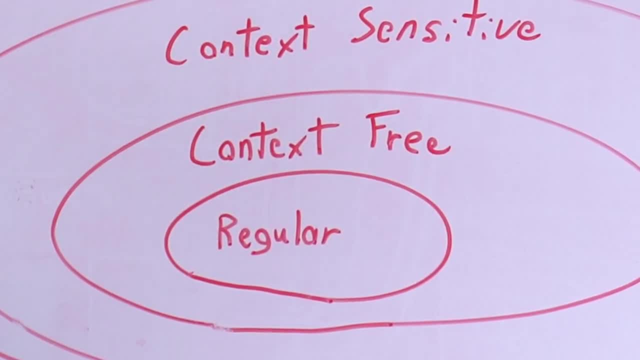 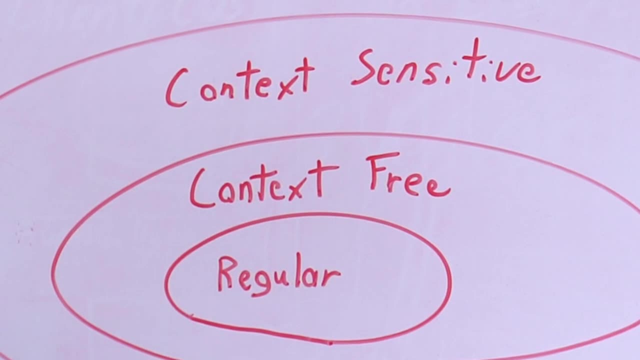 context-free languages has great practical importance. However, the distinction between context-free and context-sensitive is less profound than that between regular and context-free. And finally, the concept of recursively enumerable languages just seems like a forced attempt to extend the hierarchy to a larger set of open languages. It's a very clear picture of the 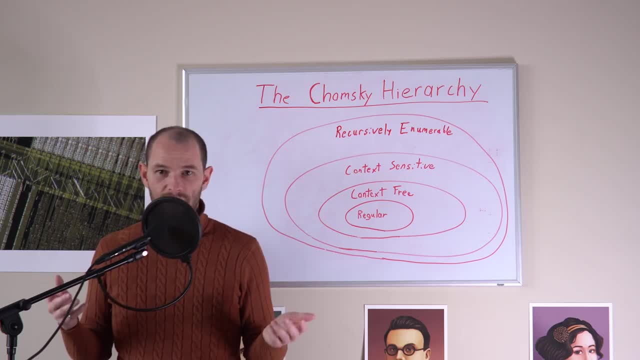 one more level just because you can. Now, I'm not trying to say that any of these models are incorrect, and I'm sure that I'll get lots of comments from people reciting back to me the textbook definition of these terms, But in a way, I think that's actually a big part of the problem. 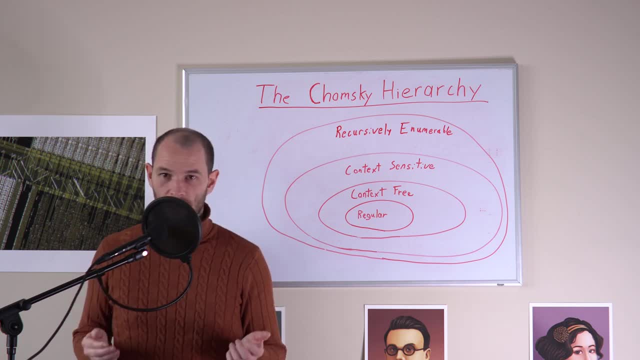 It seems like there are really two different groups of people when it comes to programming language research. One group seems to be obsessed with a form of mathematical beauty and purity that's not well connected to the real-world needs of programming languages. For this group, 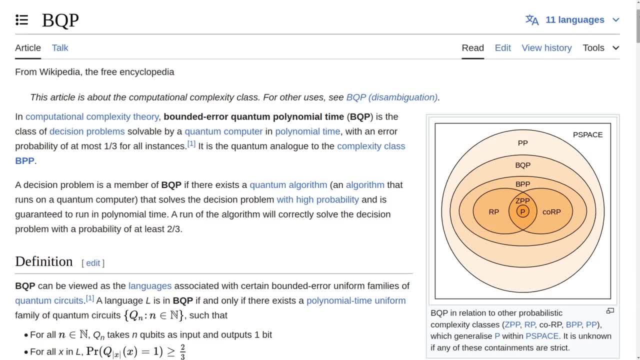 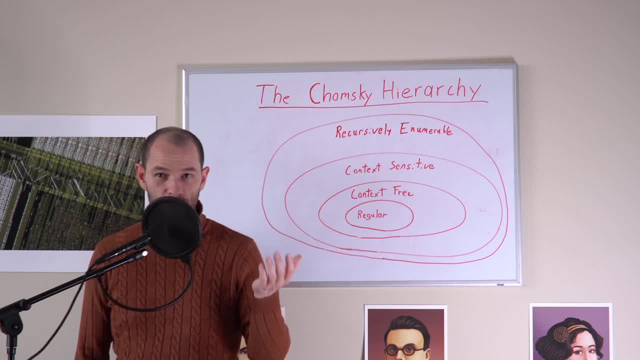 there's a relentless obsession with concepts like production rules, time-space, complexity, formal type theory and Boolean satisfiability problems. And the other group which knows about but doesn't actually use much of this mathematical purity. Instead, this group focuses all of their 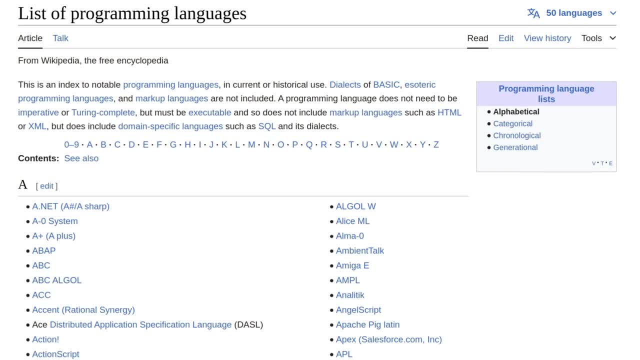 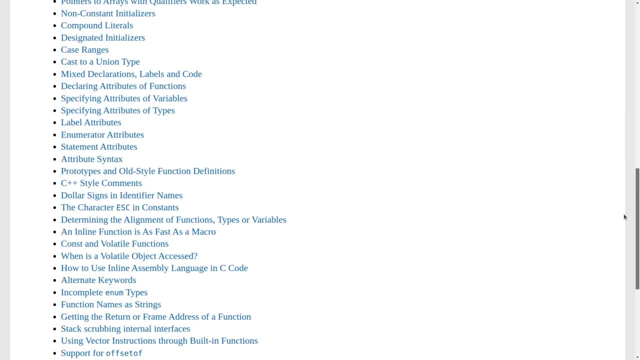 time deciding what tokens to put between statements. in their new programming language, They also spend a lot of time inventing novel pieces of syntax sugar that are marginally more convenient for programmers but incredibly hard to parse. Unfortunately, these two groups of people don't seem to talk to each other. 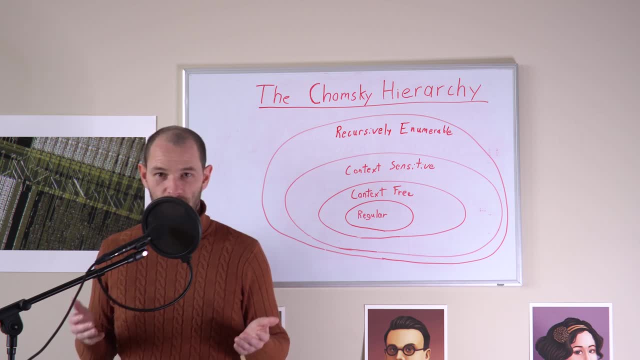 very much. If the argument that I'm constructing so far doesn't sound very convincing, let me ask you this question: If the Chomsky hierarchy is so great, why are we still writing recursive descent parsers in the year 2024?? I've come to believe that writing a compiler is a fool's errand. 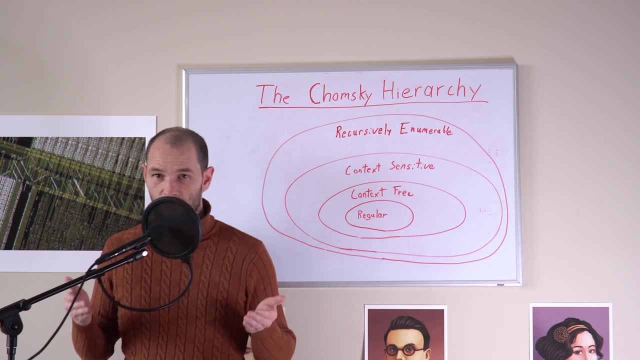 Compilers should not be written. They should be automatically generated from something that resembles a formal grammar, and not just the parser, the code generator, too. Some of you will probably argue that this is not possible, because real-world programming languages are too complicated and there are too many of them. But if you're a compiler, you should be able to write a compiler. 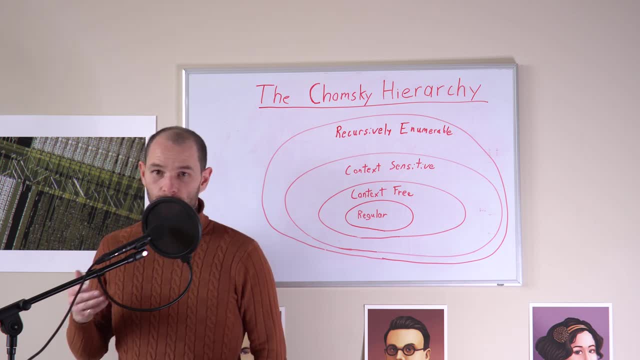 that has too many corner cases. But I don't think that this is true. I think that the real problem is that no one has done the work necessary to describe extensions to formal grammars and rule-based systems that are capable of describing modern programming languages complete with all.